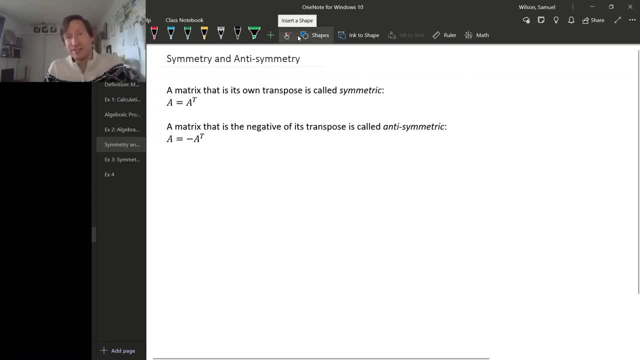 Because the matrix transpose really just reflects the entries of a matrix across the diagonal. it's possible that when you do that reflection you actually get the same matrix back. When that happens, that sort of matrix is called symmetric, So any matrix that's equal to its own. 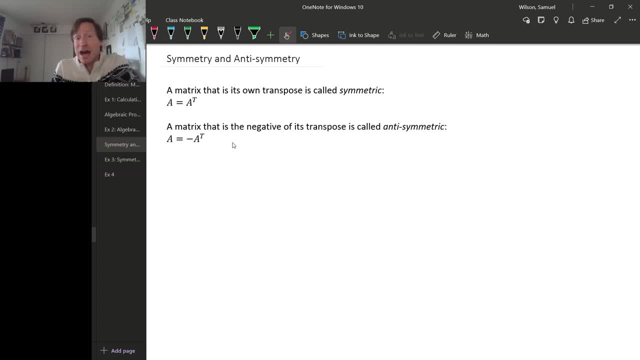 transpose is called symmetric, If you happen to get. if the transpose is actually the negative of what you started with, then it's called anti-symmetric. For both of these there are actually some size restrictions. So if A is m by n, then A transpose is n by n, m like this: 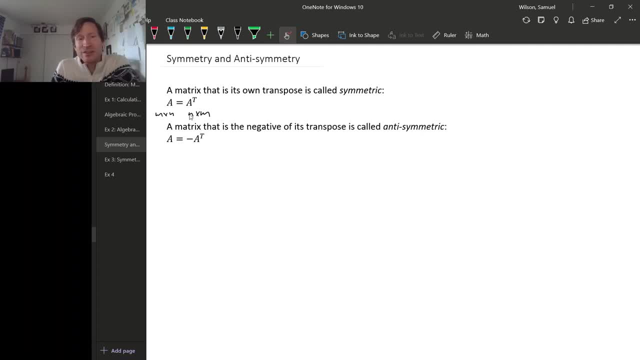 and the only way for these to be equal is if these are the same size. So m has to be equal to n for symmetric matrices. So in other words, symmetric matrices must be square, And that's actually true for anti-symmetric matrices as well. If A is m by n, that means 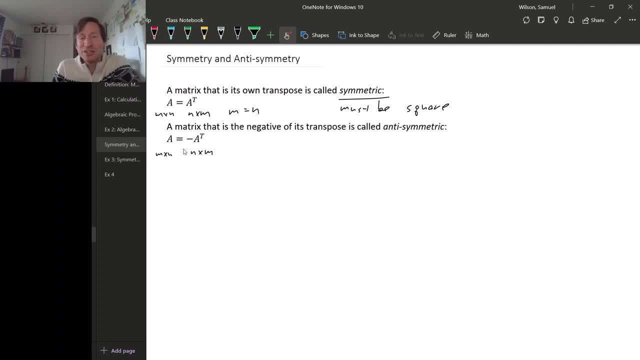 the transpose is n by m, but the only way for two matrices to be negatives of each other is if they're the same size, and that means that, right, these sizes have to be the same, and so n has to be equal to n. and again we find that it has to be square. All right, so you can only have a. 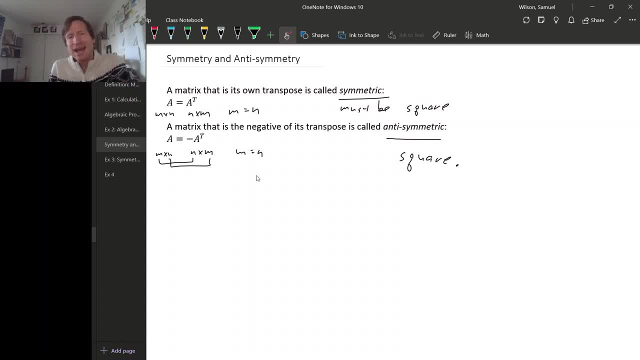 symmetric or anti-symmetric matrix if it's square and of course it has to have this symmetry property. So let's look at some examples, Let's just check whether these matrices are symmetric or anti-symmetric. So remember, symmetric means when you reflect across this diagonal. 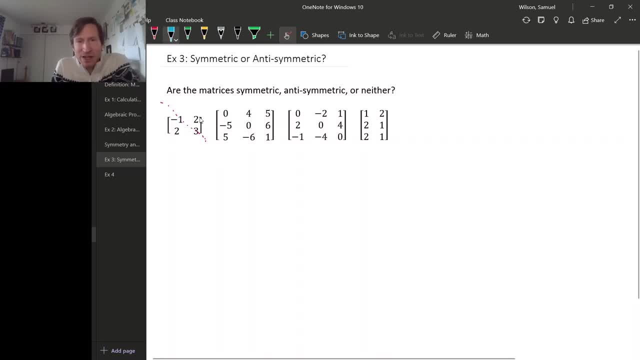 the matrix stays the same. So for this first one, when we reflect across this diagonal, the entries on the diagonal don't move, but the entries across diagonal, like this, swap places. But since they're symmetric, right, if we do this reflection, you actually get the same matrix back. So this is symmetric. 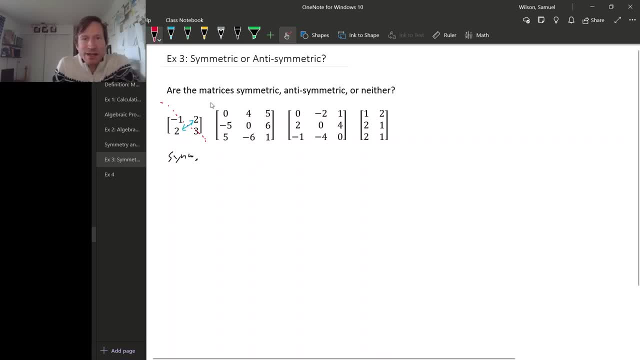 All right, what about this 3x3 matrix? So again, let's reflect. oh, incidentally, since it's symmetric, it can't be anti-symmetric. Okay, for the second one, let's reflect across this diagonal. So when 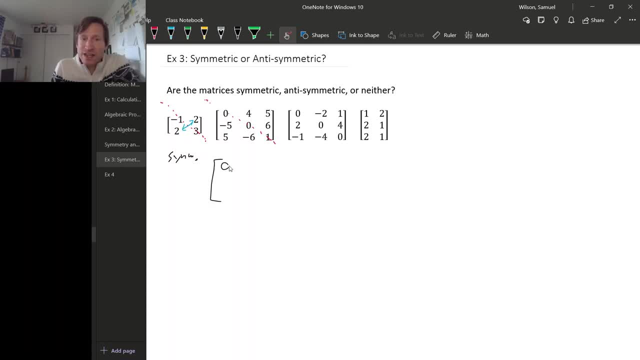 we do this reflection, let's see: the zero stays in its place, the minus 4 and the minus 5 switch and these 5s switch. the zero stays where it is, the 6 and minus 6 switch and the 1 stays where. 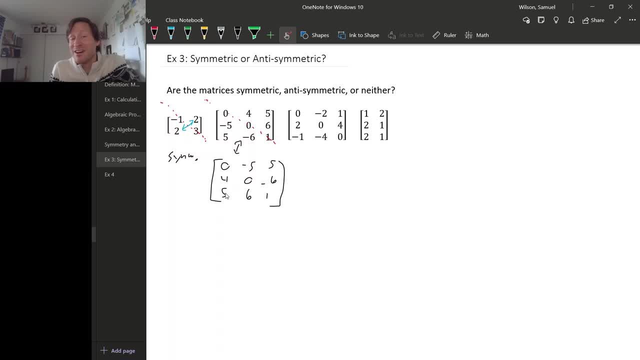 it is. So are these the same matrix? Well, definitely not exactly the same. so not symmetric. Is it anti-symmetric? Well, are these two matrices negatives? Well, no, because you know there are several entries that don't work. but just to have an example, this entry here: 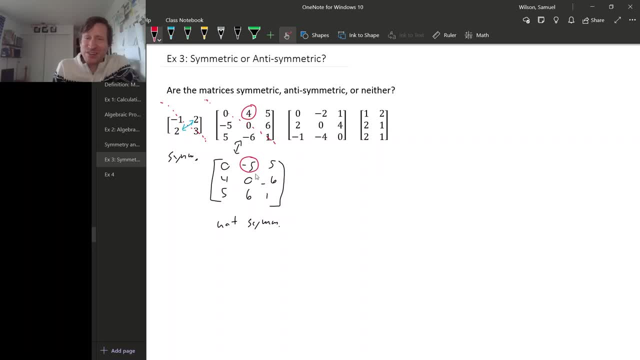 if this matrix were anti-symmetric, this should be a minus 4, but it's a minus 5.. So this isn't anti-symmetric either. All right, what about this third example? So if we do our transpose right, the zero stays put. 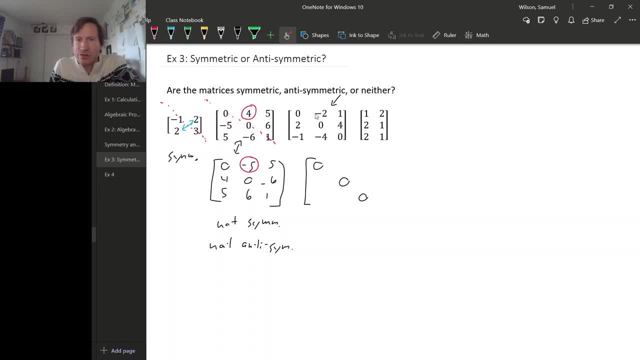 in fact the whole diagonal stays. put this: 2 and minus 2 switch places, the 1 and minus 1 switch places, and then the 4 and minus 4 switch places. okay, so these aren't the same matrix, so not symmetric. 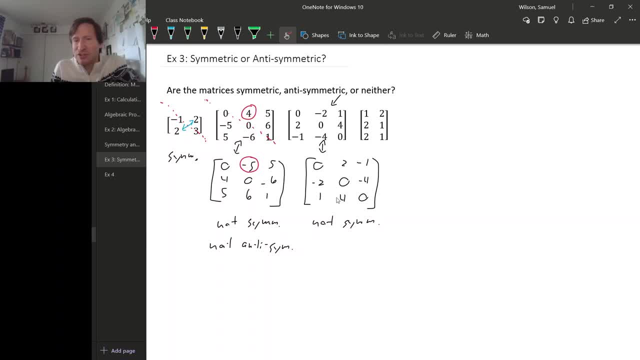 But in fact these are negatives of each other. Every entry in this transposed matrix is the negative of the corresponding entry in the first matrix. So this is an anti-symmetric matrix. Okay, what about this last example? Well, remember, we noticed that symmetric and anti-symmetric matrix 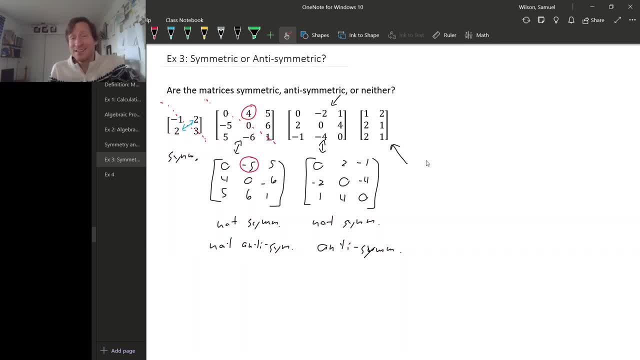 matrices have to be square and this matrix isn't square, so this is neither symmetric nor anti-symmetric. for a couple more examples of sort of what it means to be symmetric or anti-symmetric, let's just fill in some entries of these matrices in order to make A symmetric and B anti-symmetric. so for A, if we did. 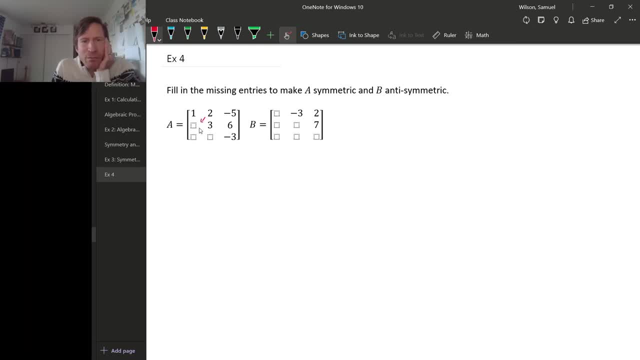 a transpose, this 2 would jump down here. but if A is going to be symmetric, that means it should have been a 2 there to begin with, so there should be a 2 here. if this is going to be symmetric, the minus 5 in the upper right would jump. 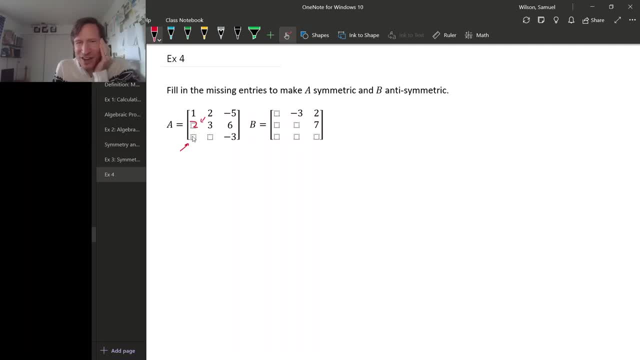 down to the lower left, but that means that it should have been minus 5 down there to begin with, so minus 5, and then, similarly, this 6 would jump down here, so we should have a 6 here. so that's how we could fill in this matrix to make it.